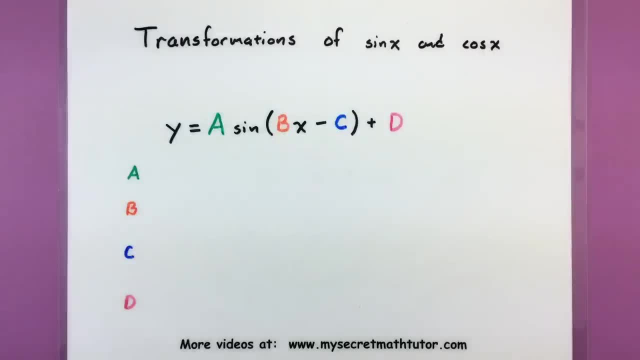 Hello and welcome to My Secret Math Tutor. For this video we're going to go over transformations of sine and cosine. So the big picture of this is that you essentially start with your basic graph of sine or cosine and you start to make some changes to it And, depending 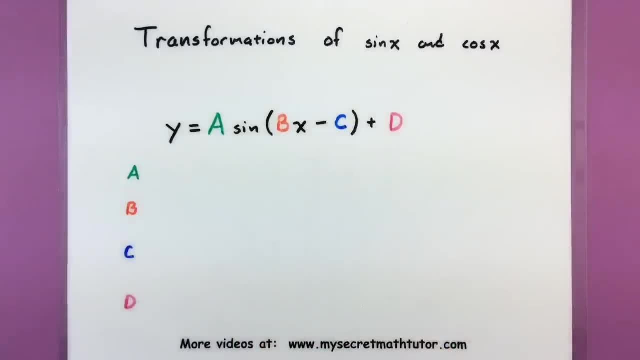 on what changes we make to the equation itself. it'll tell us how we've changed the graph of that function. So we're looking to read these key values that we see in the equation to figure out: well, how have they changed it? Have they stretched it out or maybe made? 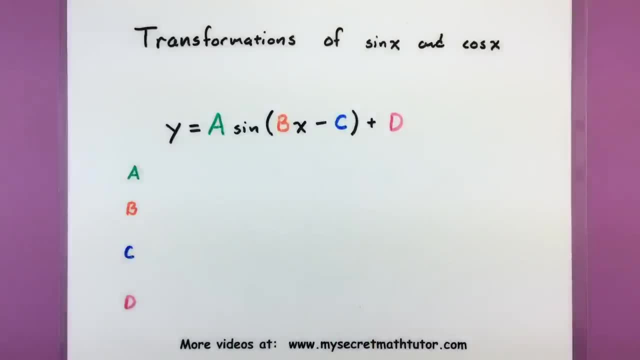 it taller or shorter, And these values will give us all the information we need. Let's cover them one at a time to see what information they have for us, and then get into some examples on actually using these things. All right, So the first value sits in front of our trigonometric 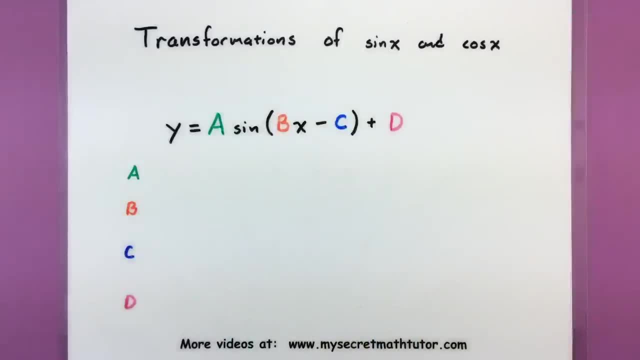 function. Again, you want to think of this as sine or cosine. It could be either one. The information is going to be the same. So the a value here, or whatever number is sitting in front of us, gives us information about the amplitude. 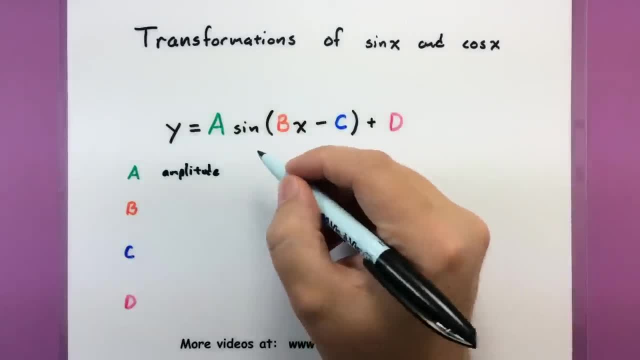 Now, I'm not saying that a is the amplitude. Usually we think of the absolute value of a that being the amplitude. Let's go ahead and just mark this as absolute value of a. Other information it gives us is whether we should flip our graph over the x-axis or not. 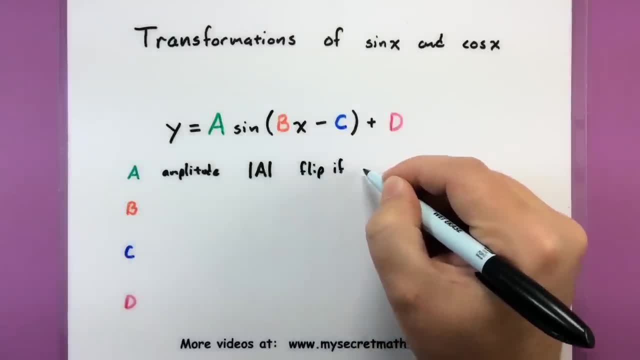 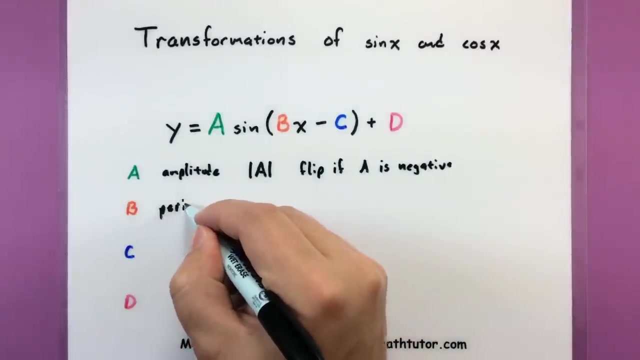 So let's say flip if a is negative, All right On to our next value. This is going to be b. on the inside, It gives us information about the period. To find the period you want to, take 2 pi, that's the usual period of sine, and divide it by the absolute value. 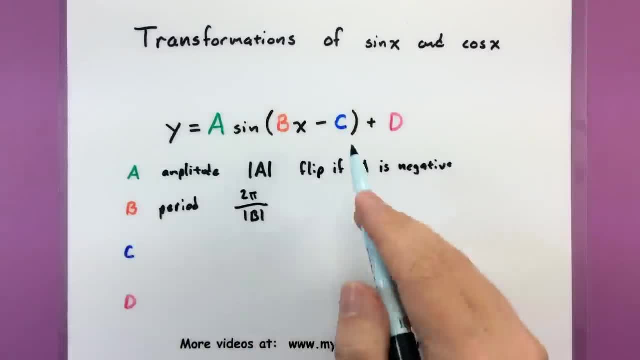 of b. c is going to tell us how far, left or right, the graph has been shifted, So this is what we call the phase shift. To find the phase shift, we want to take c and divide it by b, So we'll get most of our information from c. but really don't forget. 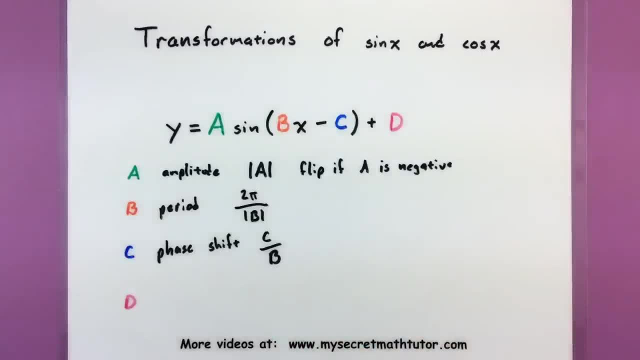 to take this one and divide it by b to see properly how far left or right has gone. Also know that there's a negative sign in here. So if this value is already negative, then we're getting information of whether it shifted to the right. If this value is a positive, 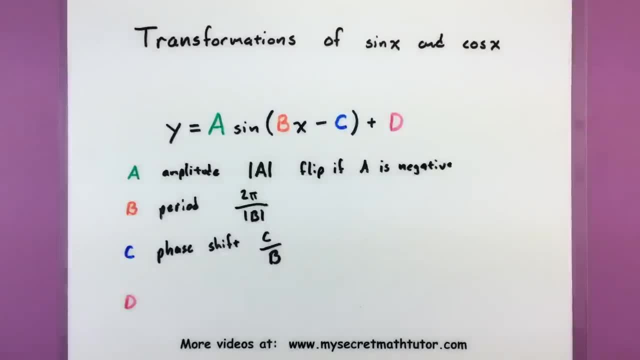 value. then we have information of how it shifted: off to the left, All right On to d. d is for our vertical shift. So this is telling us how far up or down the graph has been moved, and this is just the value of d itself. All right, So now that we know a little bit about each of these parts. 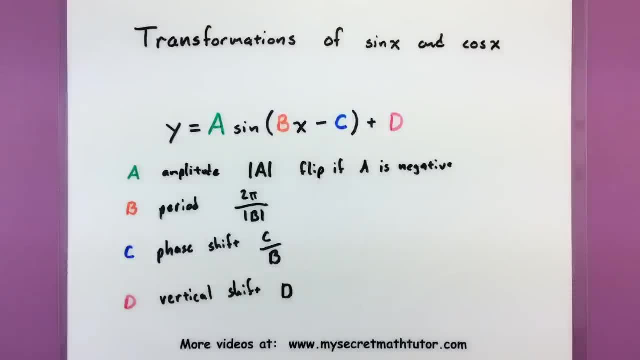 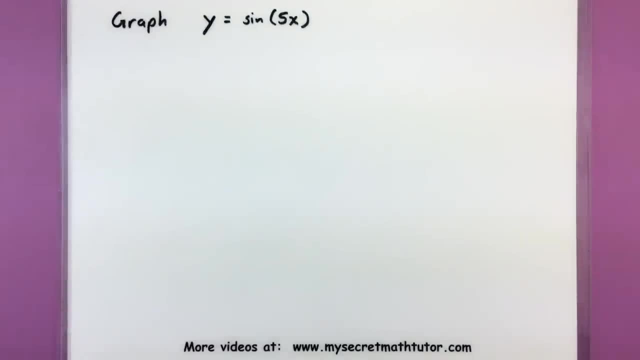 let's get into some examples and start reading these so we can go ahead and make a nice graph of one of our transformed functions. The first of these will be graphing: y equals sine of 5x, And before we actually get into the graphing part, I'm going to show you how to do that. So we're going to go ahead and 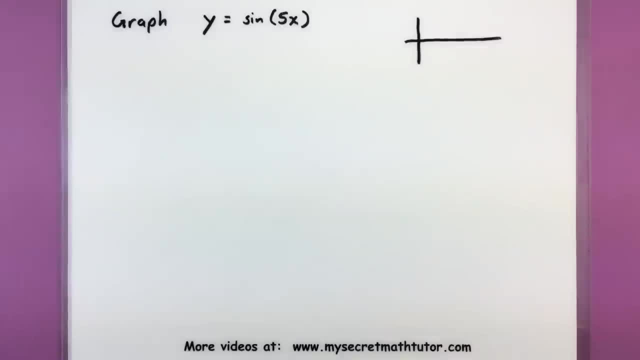 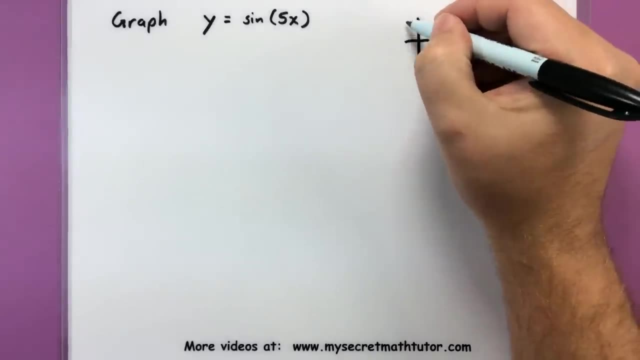 do that. A good habit is to just keep the basic function of what sine looks like in the back of your mind. That way you can refer back to it and say: okay, if that's the original, what have they really changed? So in the original we would have an amplitude of 1, and we would have a period of 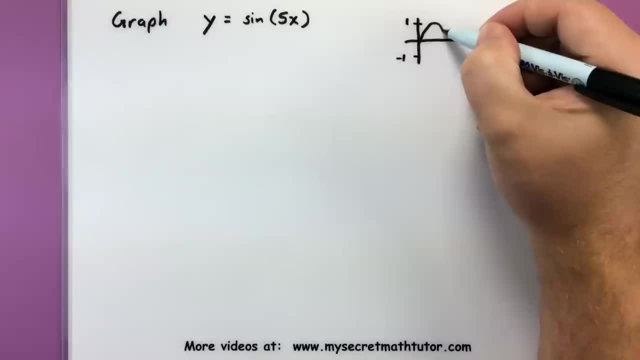 2 pi. And, of course, sine is that nice little s-shaped curve. It looks like this: We'll only draw one period, but it does continue on in both directions. So I'm thinking about this basic shape as I go to make this one. All right, Let's list out all of our values. 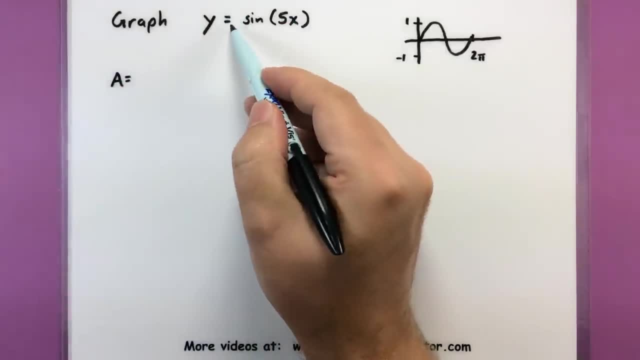 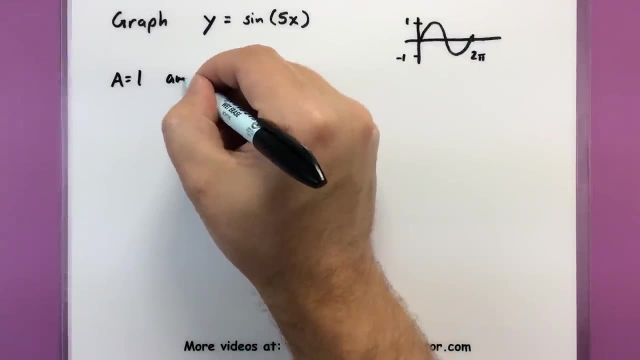 A is the number that sits in front of our trigonometric function. In this case it is 1.. So we're going to use that to read our amplitude. We're thinking of the absolute value of A or in this case, our amplitude is just 1.. 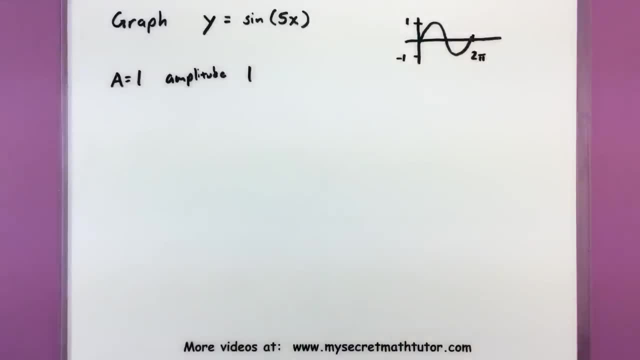 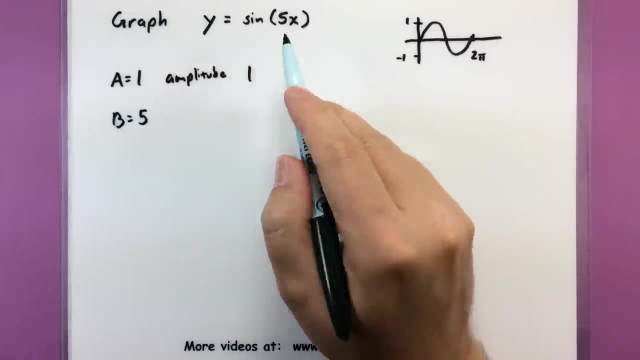 So it hasn't been stretched to make the peaks any taller or lower. On to B. B is the value that's sitting right next to our x, And in this case it's 5.. So that's going to give us information about the period. 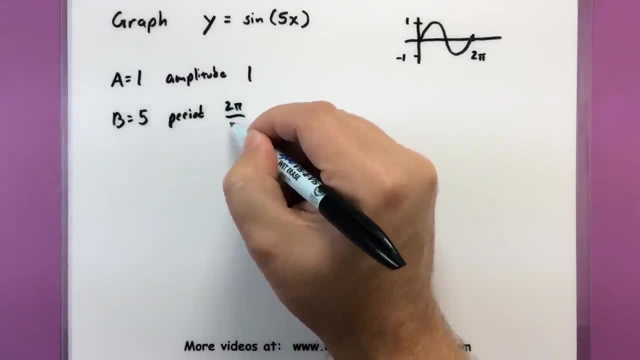 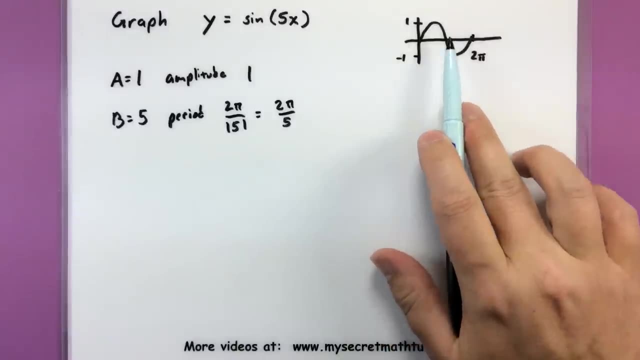 To find the period. remember we're going to take 2 pi divided by the absolute value of 5.. So we'll just get 2 pi over 5.. This means that the usual graph cycles in a period of 2 pi. It. 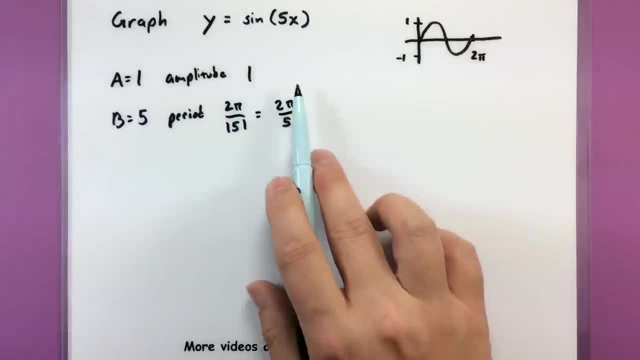 goes through one complete period, Whereas ours it's not going to take quite as long. It's going to go through that one complete period and only 2 pi over 5.. All right, Let's see what else we got. C and D. So C would be the number that's subtracted over here. There is none. 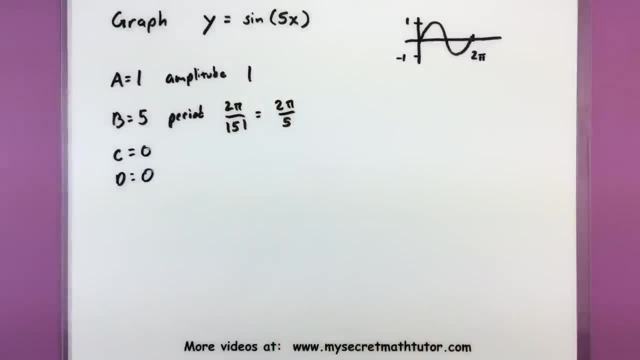 And D would be any numbers added or subtracted to the outside. There is none of those. So it tells us that we have no phase shift and no vertical shift. It hasn't been moved left or right, or it hasn't been moved up or down. So now that we've got this basic information out of the way, 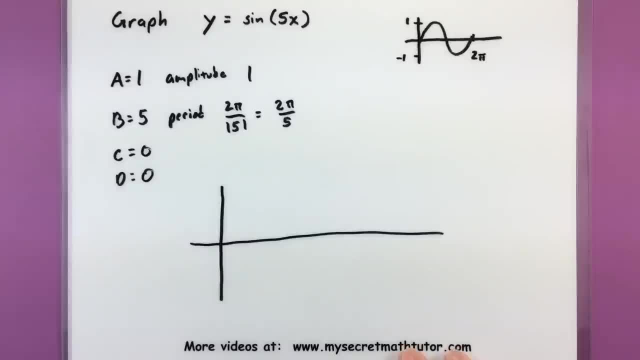 let's go ahead and graph our brand new function and see what it looks like. So I'm going to start off with the amplitude. It's simply a 1.. So it's going to be the same amplitude as our original. So 1 and negative 1.. The period is what is changing. So, rather than going between 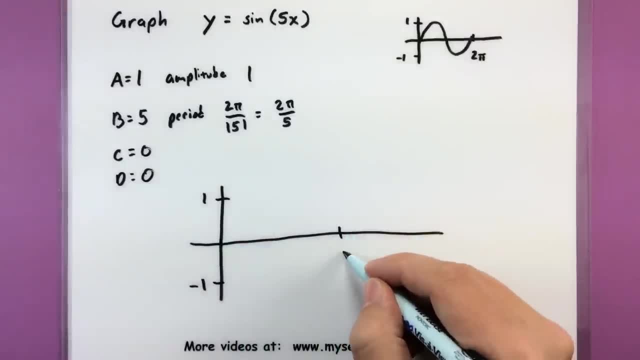 0 and 2 pi. we want to imagine this going between 0 and 2 pi over 5.. Not bad, Everything else is 0, so we don't want to move this left or right or up and down. So now let's just draw in one nice. 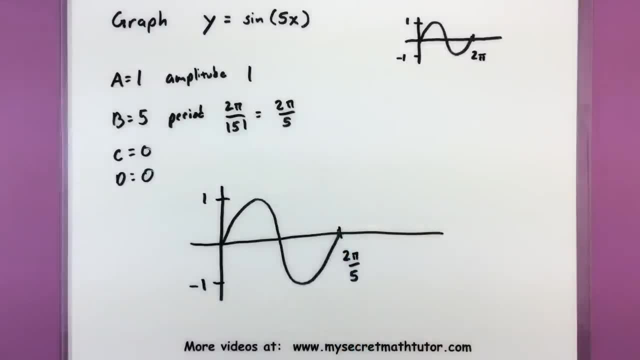 complete cycle. There we go, So that would be a nice simple graph of what sine looks like. If you're really curious, like hey, I think I need some more key values in here, remember the halfway point is going to be, or where it crosses the x-axis is the halfway point. 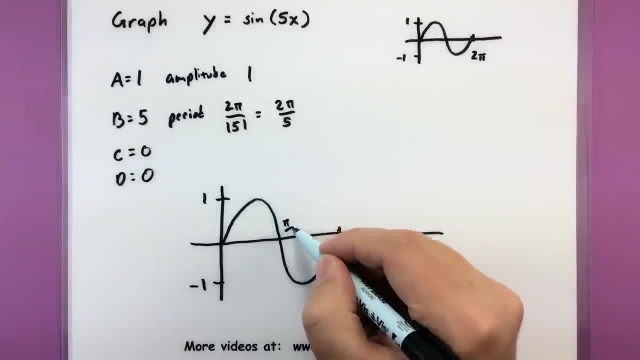 So you can take 2 pi divided by 5, chop that in half and that'd give you just pi over 5.. If you chop pi over 5 in half again, then you'd get a couple more key values. This one would be at pi over 10.. 2 pi over 10.. This one would be at 3 pi over 10.. 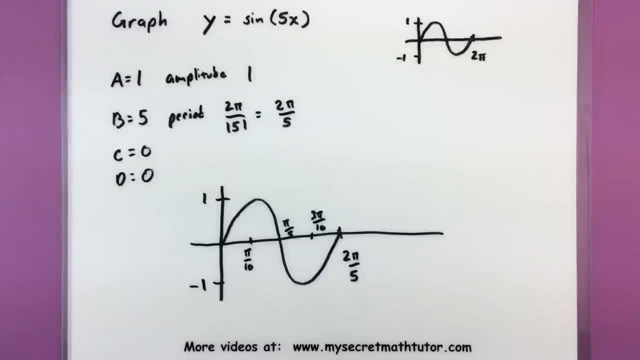 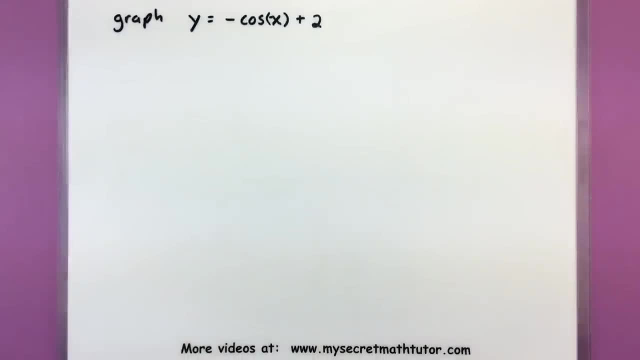 And 4 pi over 10, or 2 pi over 5.. So just some things you can write down. All right, let's see another example. Let's make this one a little bit more difficult. This one involves cosine. So in the back of our mind, let's get a nice basic graph for cosine. 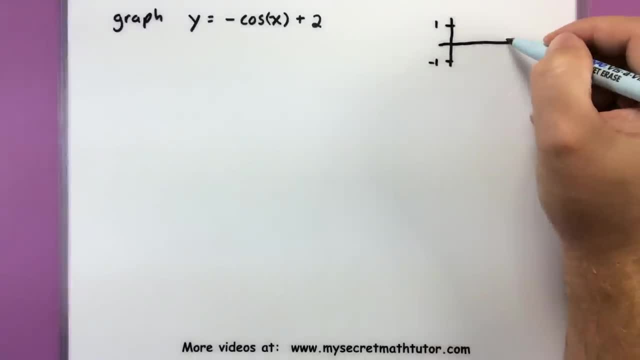 We have our amplitude of 1, a period of 2 pi And cosine. I almost like to think of it as a u-shape. I know it's not a u-shape. It really does, you know, look like sine, but it's a u-shape, So I'm 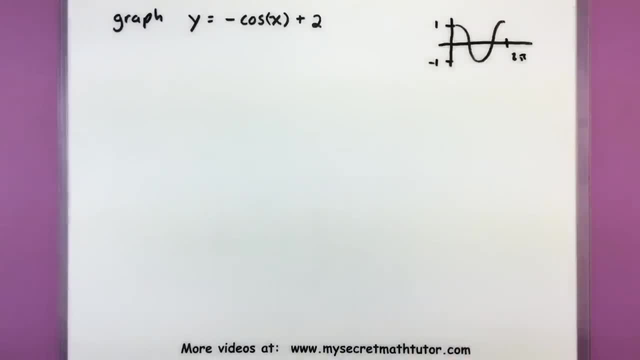 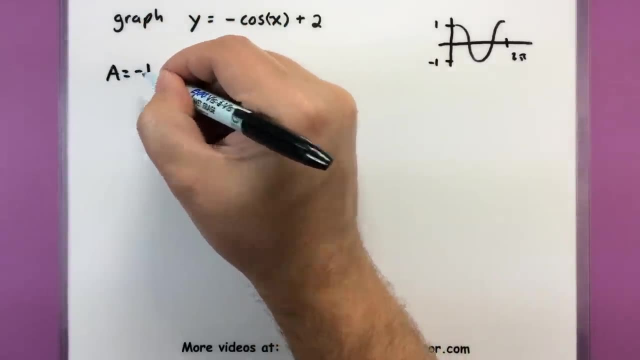 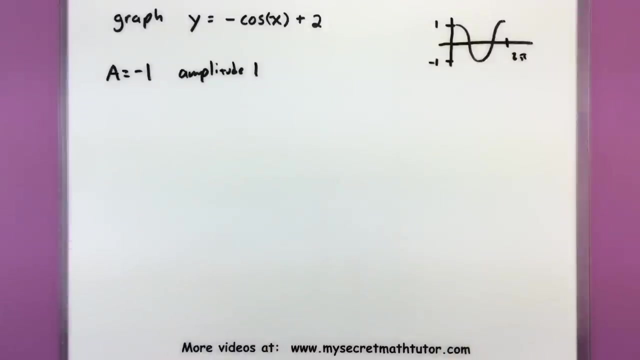 going to go ahead and get my amplitude dyred. This one's going to be us. Omega will be equal to k. These two come together. I'm going to come in half and I'll just06 нибудь a吸. 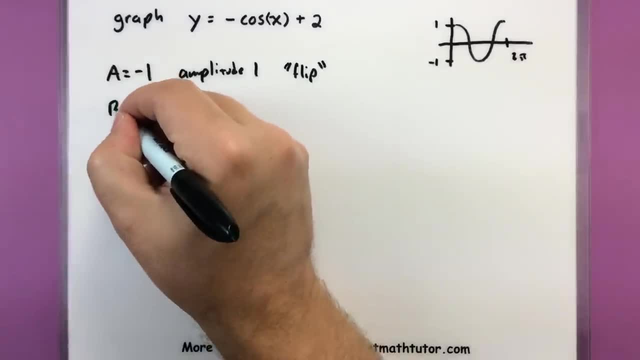 ok, so that's just 1 pi divided by 2 pi. That's better. I know that works out pretty good. All right, on to graphing this thing. So A in our case is the number that sits out in front, negative 1.. So our amplitude is going to equal 1, but the negative tells me I should flip this over the x-axis. All right on to B. b is the value next to x and I'm going to make a little note that I need to flip it. 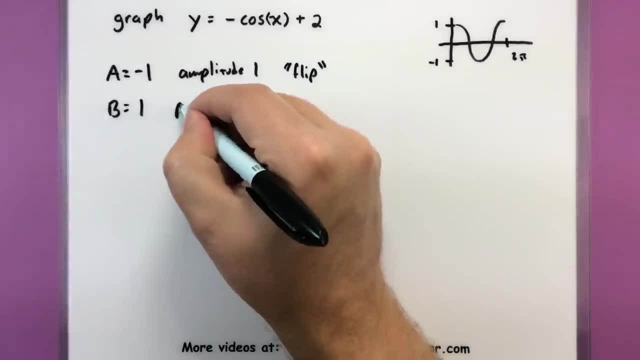 All right on to B. b is the value next to x, and I'm going to make a little note that I need to flip it same thing, so we will assume that is one. so our period is two pi over one or just two pi. 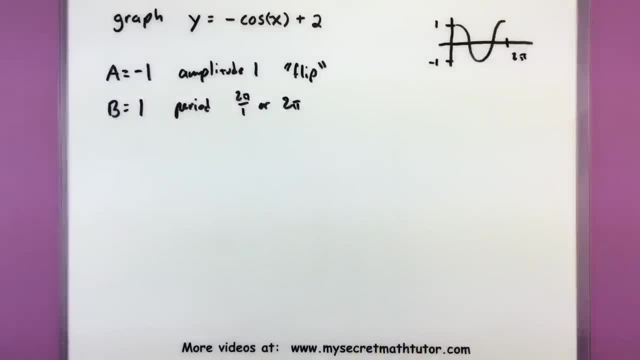 that means it has the same period as our basic function for cosine nice c. c is uh, the number on the inside there- um that is added or subtracted. i don't have any numbers, so there is no phase shift. moving on to d, it looks like we do have something that is added. 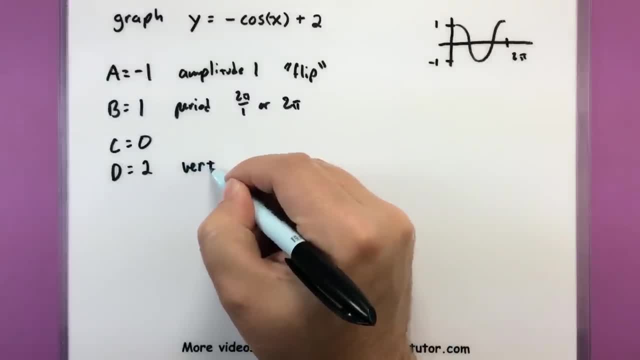 on the outside. so d that will be our vertical shift. so everything's been moved up by two. okay, so we got some good information. let's draw out this graph. i'm going to start way down here, on the bottom, with the vertical shift, because it'll give me a sense of where i'm going to center things around. 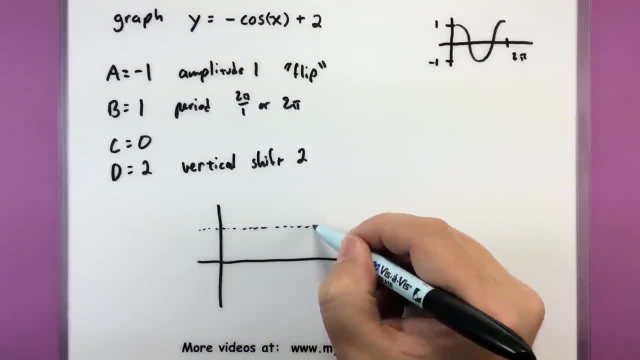 so everything's been moved up by two. i'm going to use this dotted line to remind myself that, sure enough, things have been moved up by a factor of two. you want to think of this as your brand new x-axis when you're building things moving on to our amplitude. so if i go up from here one and down below one. 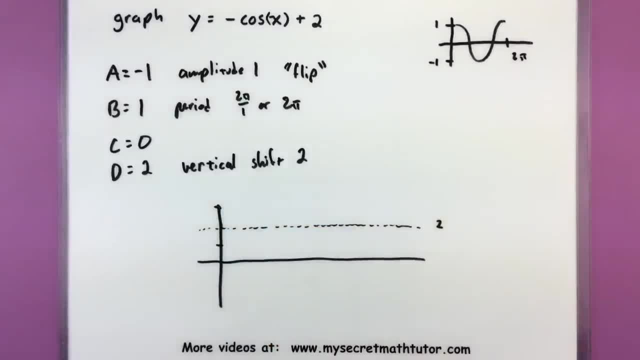 i will find the peaks and valleys of our new function. so we're at two up, one would be at three down, one would be at one. so now i have the maximum and minimum. okay, that's looking good. we don't have any phase shifts, so i'm not going back and forth and the regular period is just. 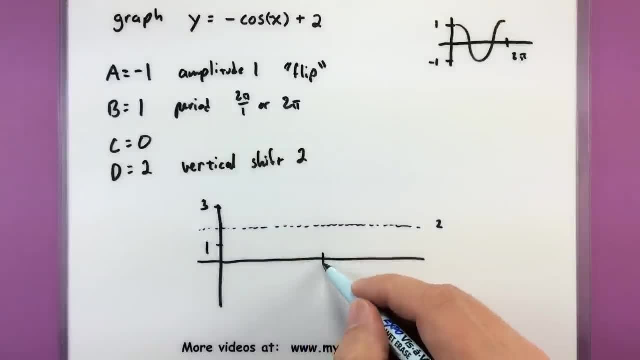 a two pi. so it goes through one complete cycle: two pi looks like we have a note here. we need to flip the graph over, so rather than making our shape like this, we're actually going to flip that over and make it upside down. so, upside down, u shape more like that. 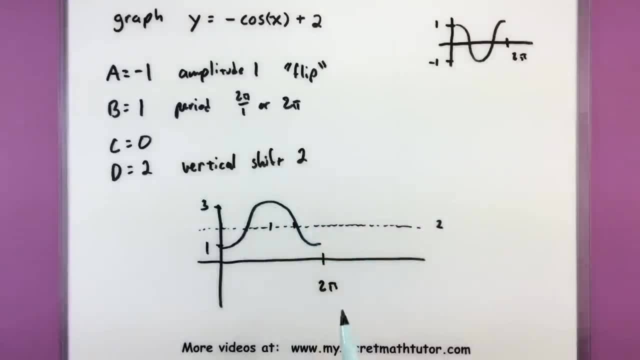 now I last. I probably want to put on some key values. so halfway in between, this would be two pi divided by two, so there's pi, and then chop that in half again and I get some more key values at pi over 2, 2, pi over 2,, 3, pi over 2, and now I have my graph for negative cosine of x plus 2.. 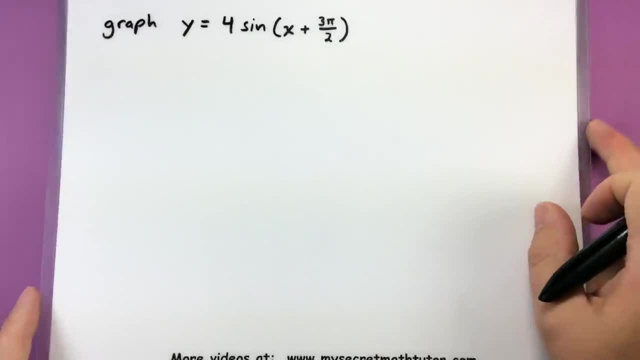 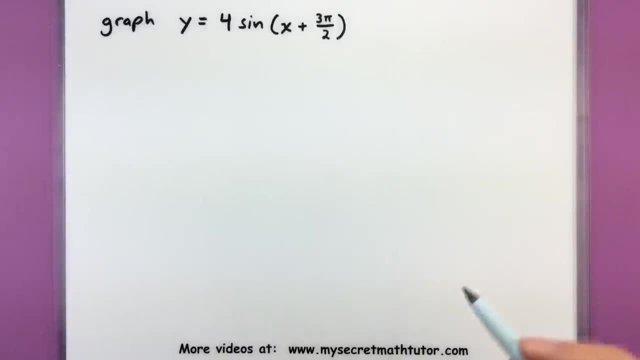 Okay, let's keep throwing in some more values and get some more difficult graphs. Moving on: y equals 4 sine of x plus 3 pi over 2.. So basic graph 1, negative 1, 1 period and 2 pi. 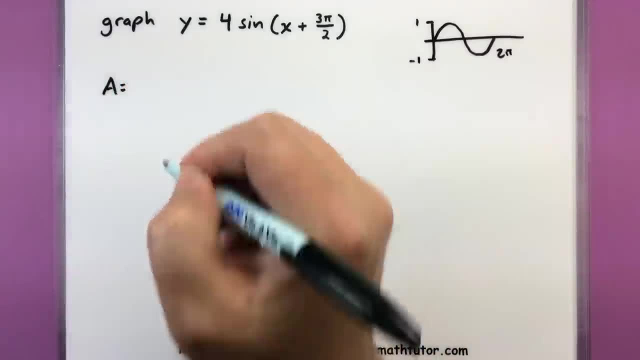 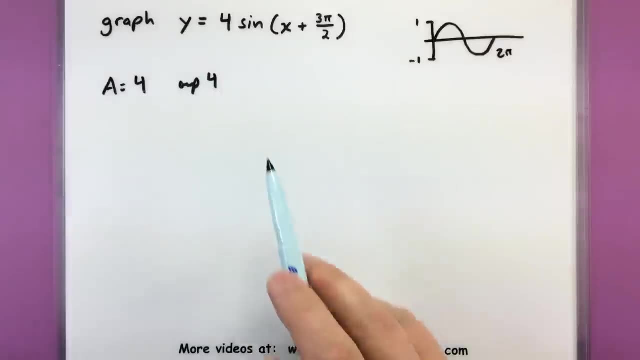 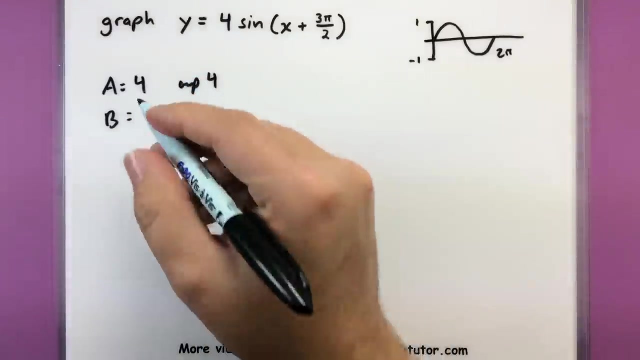 Okay, we're going to keep that in the back of our mind. Moving on amplitude Looks like our amplitude is just going to be 4, and we're not worrying about flipping anything over. since it is nice and positive B, I'm going to look in front of x to see if there's any value there. 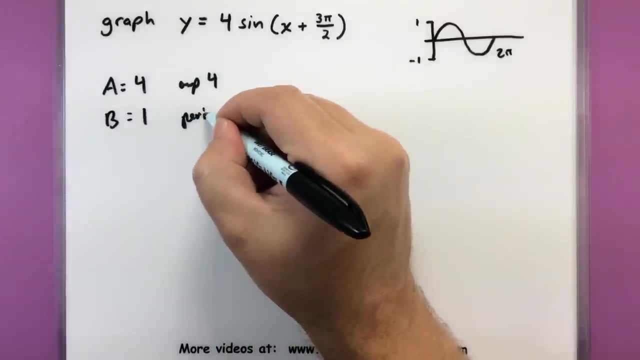 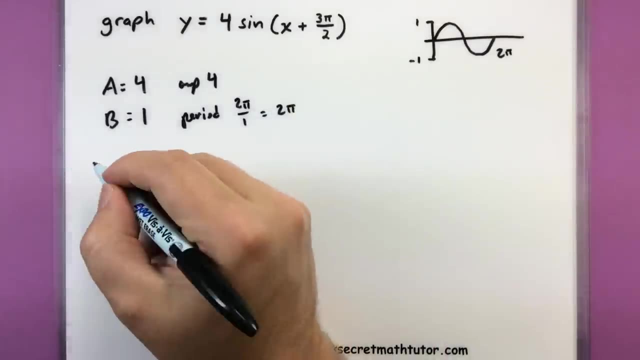 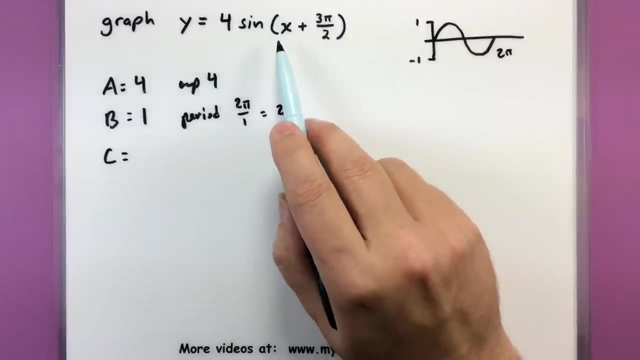 We have a value of 1, so our period, it's just a regular period divided by this value, or 2 pi. Okay, that looks good. C, C would be whatever number this is, or you'd really want to think of it as x minus this number. 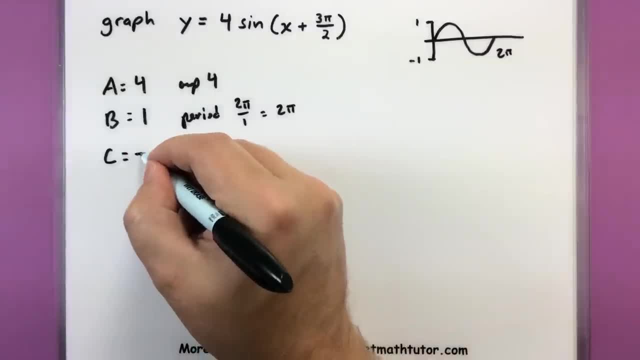 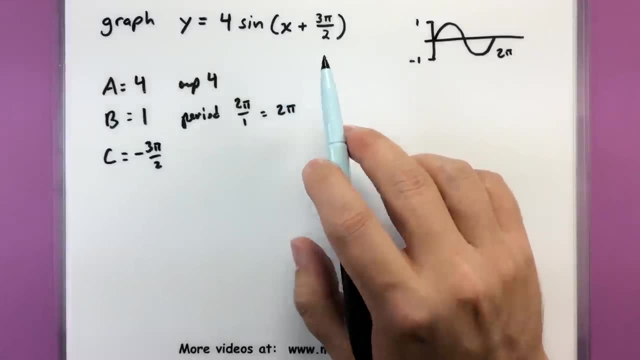 That's our value of C. Since it's positive, I'm going to mark this as negative: 3 pi over 2.. So what I'm visualizing here is x minus a negative 3 pi over 2.. That way I can get my proper value. 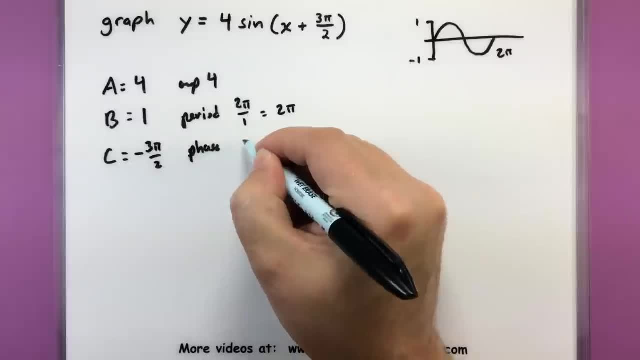 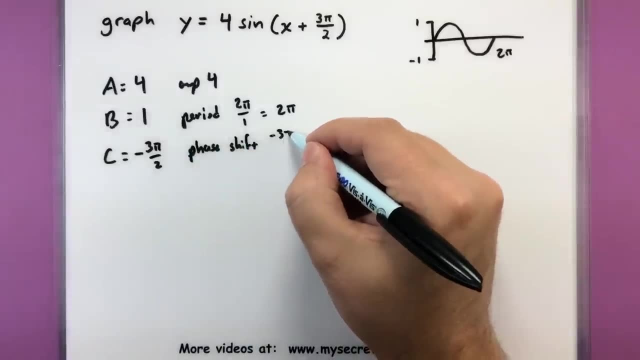 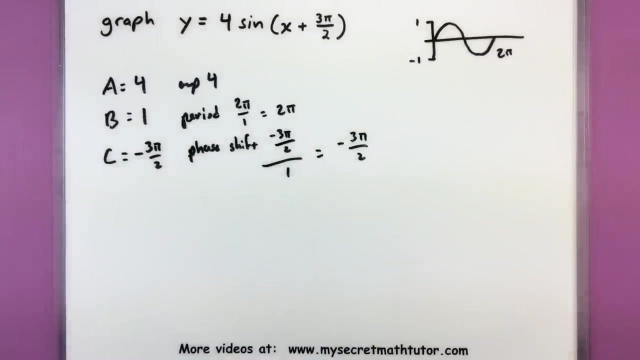 So phase shift We'll come from taking our C value and dividing it by B, So negative 3 pi over 2, all of that's being divided by 1, so just negative 3 pi over 2.. That tells me that, rather than starting at 0 for my regular graph, 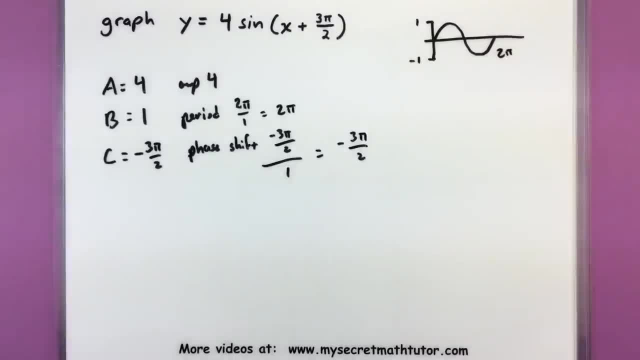 I'm going to truck it over to the left and it's actually going to start at negative 3 pi over 2.. Alright, let's see what else we got. So we have our D, We have our vertical shift. that's up and down. 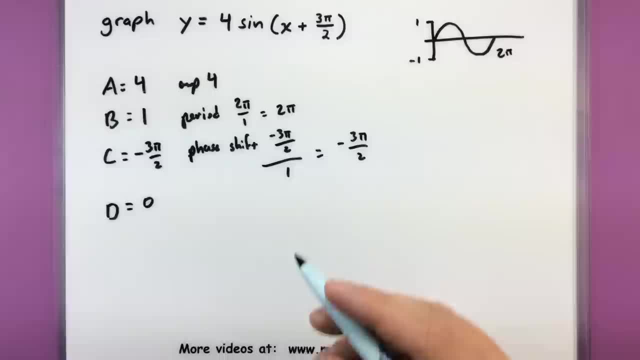 I don't have any vertical shifts, so that's just 0.. Alright, let's see what this graph looks like. So we don't have any vertical shifts. We're not going up and down any, so I don't have to worry about that. 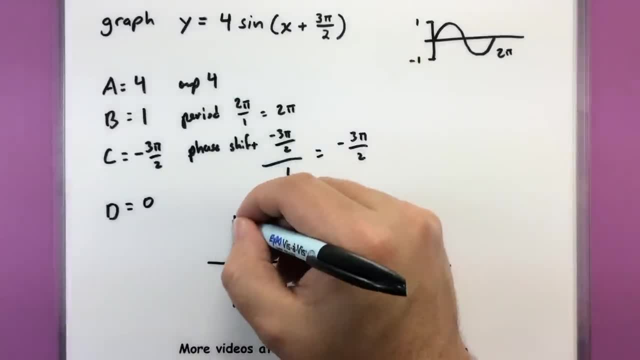 Let's see onto the amplitude. Amplitude is 4, so we'd mark that out as the little maximum peak and the little minimum peak For our sine. we know that this will cycle through in exactly 2 pi, but we're going to start it back a little ways. 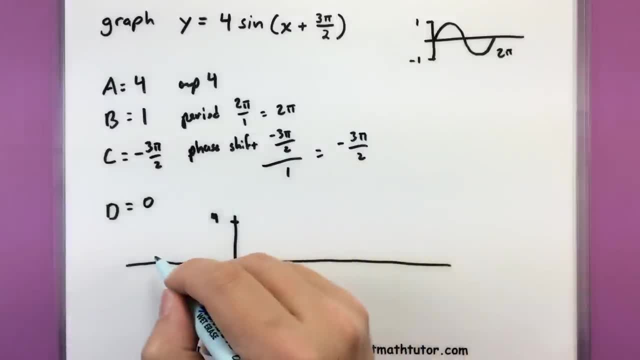 We're going to start it back here at negative 3 pi over 2.. So negative 3 pi over 2.. So that's where it actually starts. Now, if that's where it starts, and then it runs through a cycle. 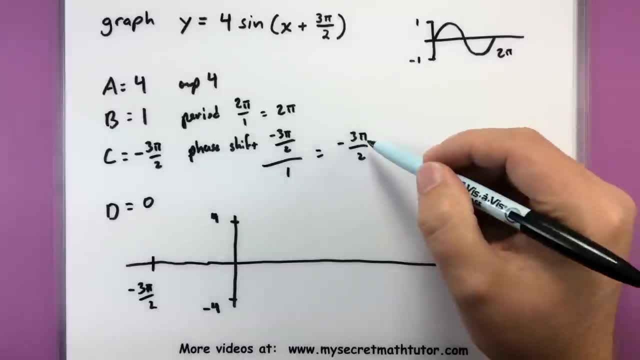 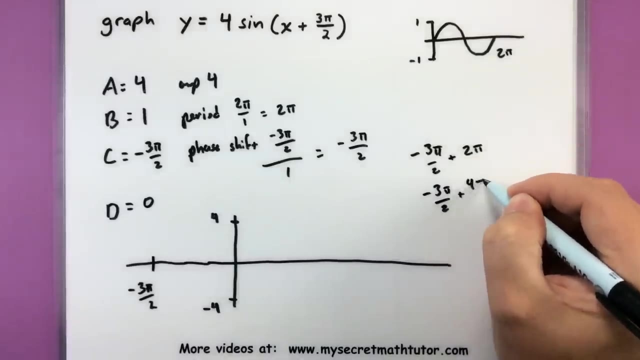 I really want to know where it should stop, And I can figure out where it stops by looking at the phase shift and just add one period in there. So 3 pi over 2 plus 2 pi, Or I could say 3 pi over 2 plus 4 pi over 2,. 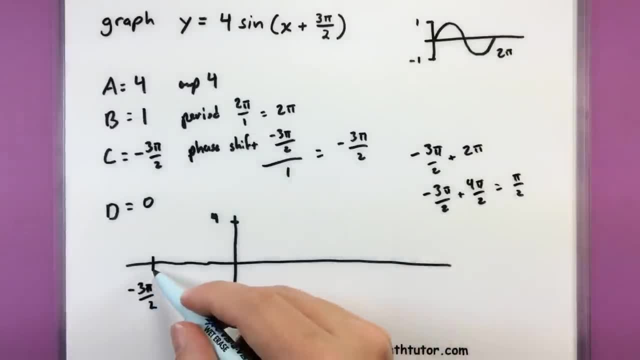 which is just equal to 1 pi over 2.. So it'll make one complete period and then I can show it ending that one period at pi over 2.. Alright, so if I had to chop this into quarters, let's see. 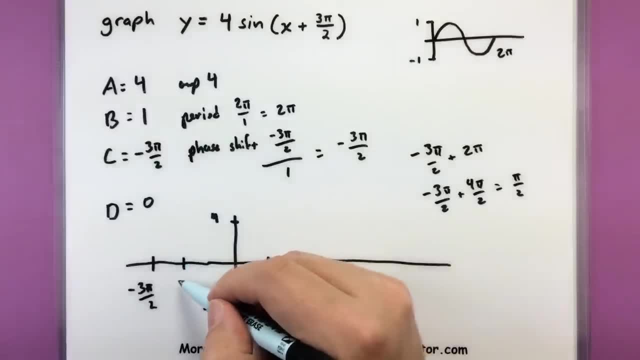 What'd I get? So I'd get negative 2, pi over 2.. Negative pi over 2, then I'd be at 0. And then pi over 2.. So 1,, 2,, 3,, 4.. 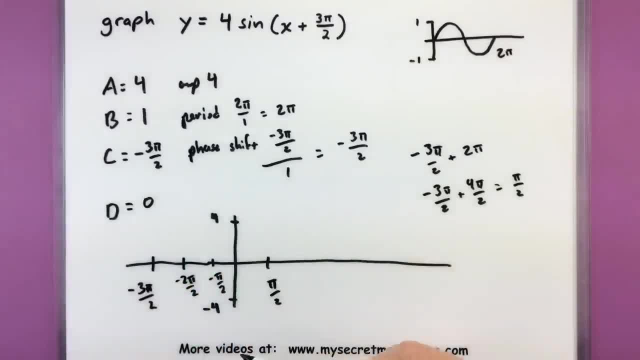 Okay, that works Alright, let's go ahead and draw our cycle. So this is for sine. So I'm starting at the x-axis. We will go up, reach our peak for our first little quarter there And we're going down. 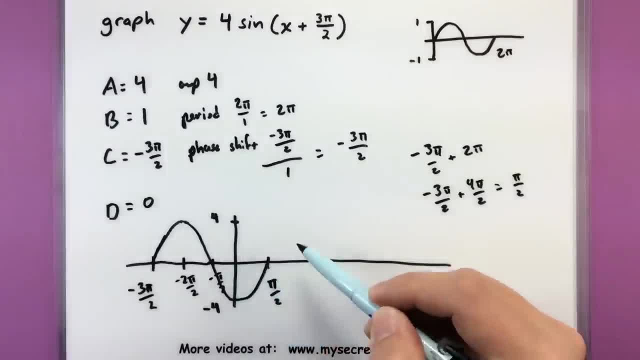 Crossing the x-axis, there's our bottom peak and ending there, And of course it does continue on, but we'll only draw just this one period. Alright, not bad. Let's see one more example, just to make sure that we have this process down. 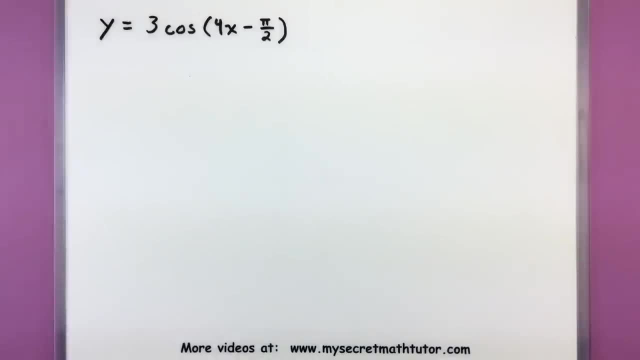 Alright, this one we want to do. y equals 3 cosine of 4x minus pi over 2.. Basic graph 1, negative 1, cycle of 2 pi Cosine. I'm thinking of this u-shape. 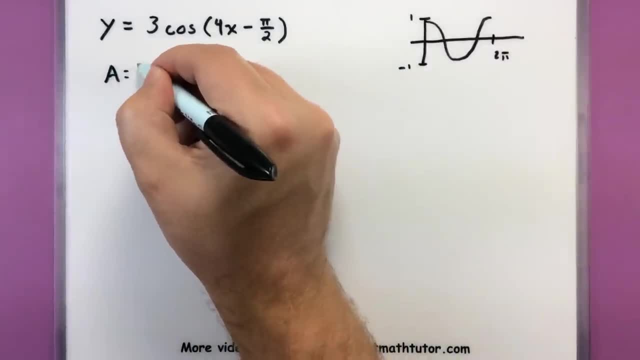 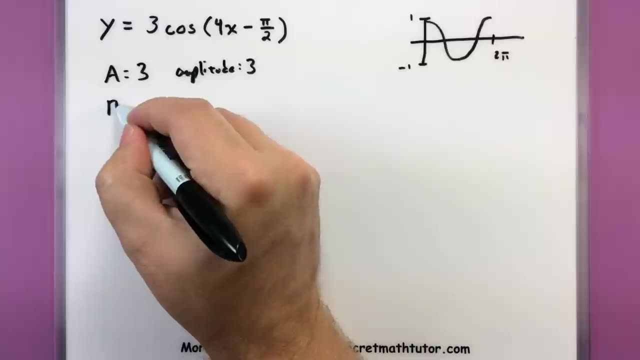 So something like that. Okay, looks good. a is equal to 3, so that's our amplitude 3.. We have a number in front of x. This is 4. So we're going to use that to find our period. 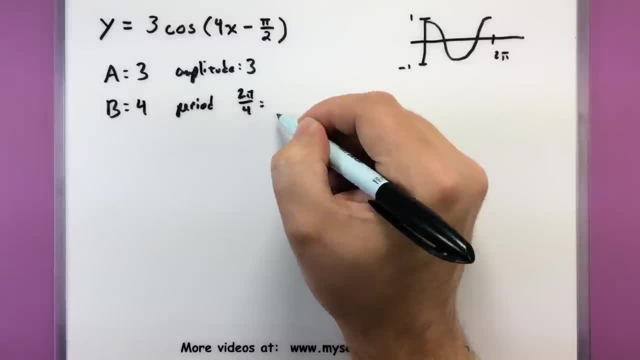 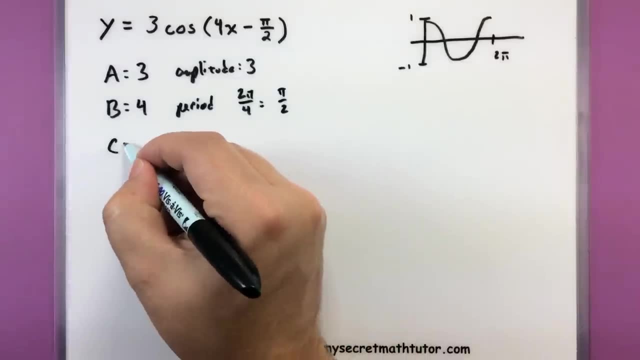 2 pi divided by the absolute value of 4.. Or in this case, just pi over 2.. So we'll make one complete cycle in pi over 2.. Okay, that's looking fine On to c. c is pi over 2.. 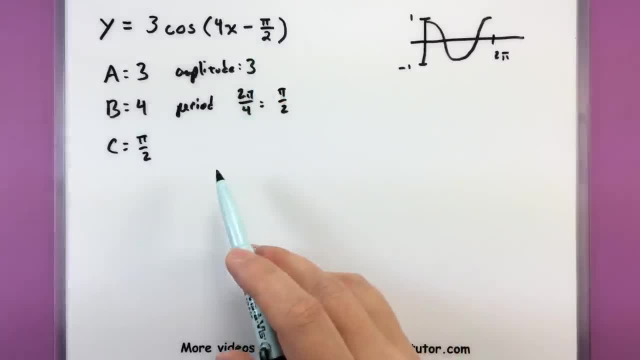 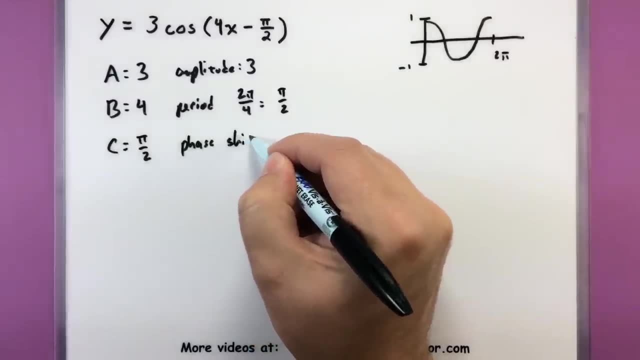 Notice how, in this case, I'm not taking the negative sign, because it already has the negative sign in there. So just pi over 2.. So our phase shift. We will take this pi over 2.. We're going to divide it by b. 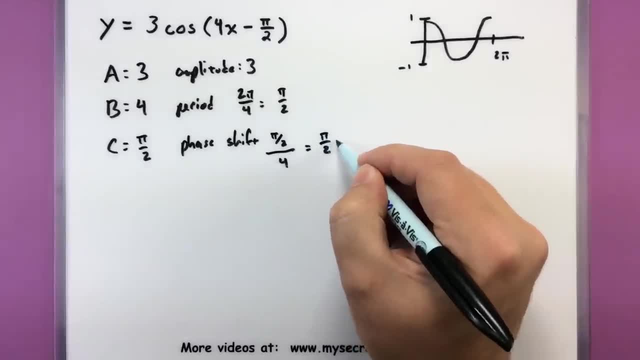 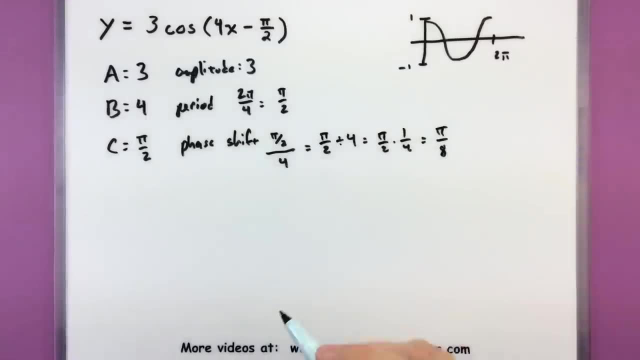 So we're going to divide this by 4.. So pi over 2, divided by 4, which is pi over 2, multiplied by 1, fourth, which is pi over 8.. So we're going to start this. 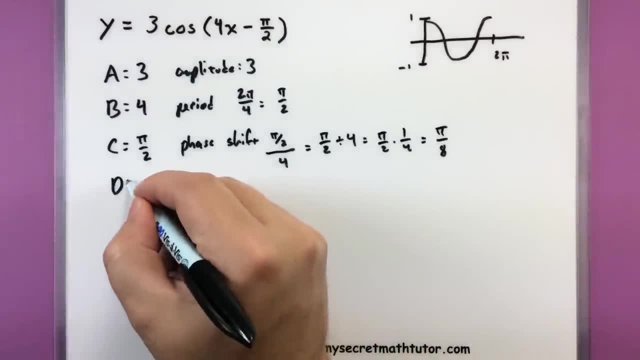 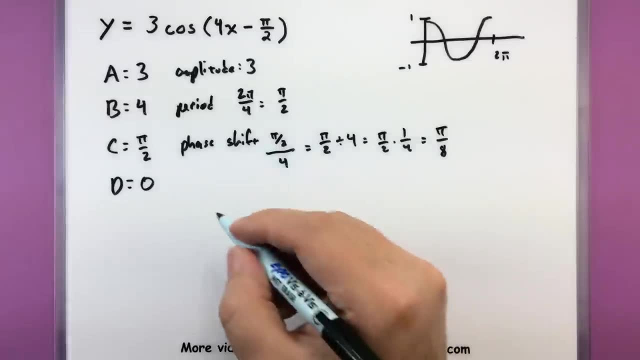 or we're going to move it over pi, over 8.. And d? this is if it's been moved up or down. This is our vertical shift. We have 0, so there is no vertical shift. Alright, we have all the information we need. 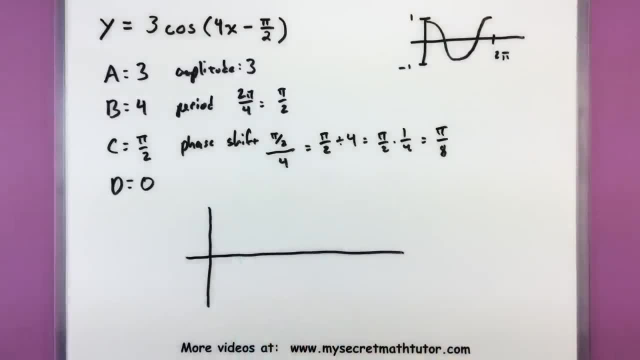 Let's go ahead and graph this, So we're not moving this up or down. I don't have to worry about that. Amplitude is 3.. So I know I'll reach a peak at 3 and a valley at negative 3.. 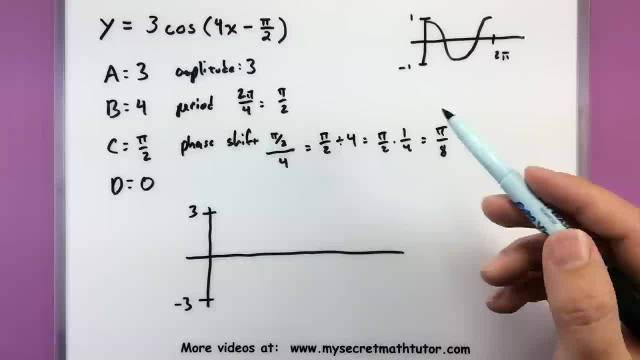 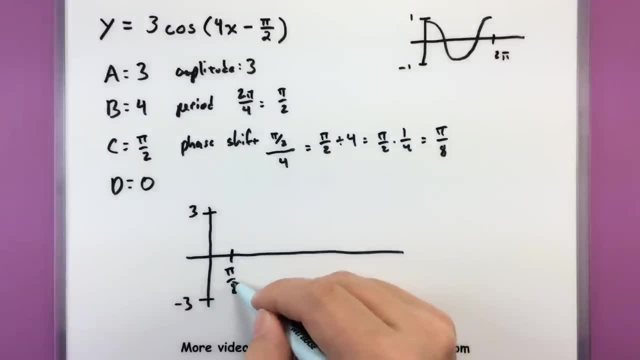 That's nice. I'll make one complete cycle at pi over 2.. But if I want to start drawing what these periods look like, I'm going to draw my first period starting at pi over 8.. So I'm thinking of the basic shape of cosine. 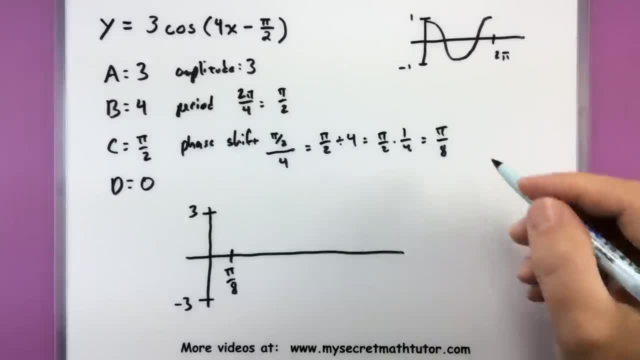 I need to know where I can show this period stopping. So I think of taking pi over 8 and I add one complete period to it. Our period is pi over 8.. So pi over 8 plus, let's see 4 pi over 8,, 5 pi over 8.. 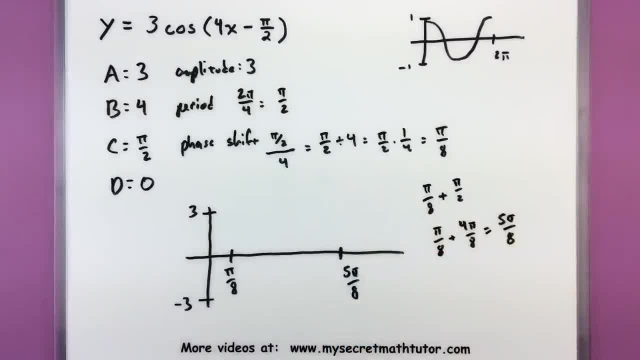 Let's put that over here at 5 pi over 8.. Alright, so I don't see anything else on there, So I want to think of where it starts. It reaches its minimum value halfway through and I'll go back up here. 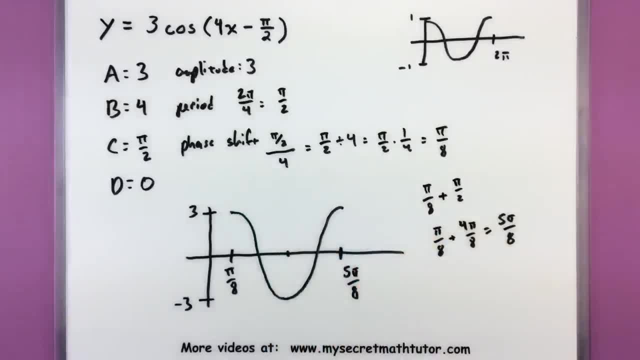 I can draw that nicely. I'll give it a nice U shape and then that looks pretty good, And of course it does keep going on. It's always good to emphasize that. you know this will make even more of these periods. 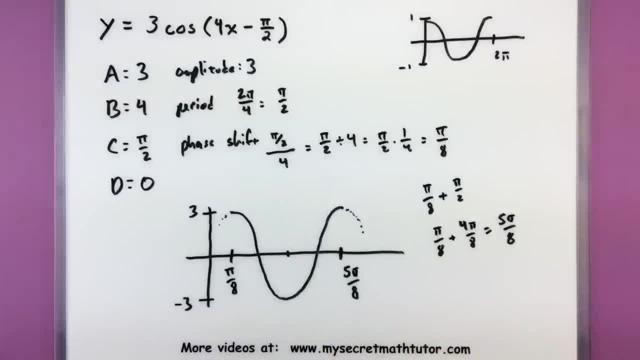 as we continue in either direction. But we'll just draw one and understand that it does keep going. Alright, it'd be nice to have some more key values in here so I could figure out where this like halfway point is. I could subtract these two so I know the distance between them is actually just pi over 2.. 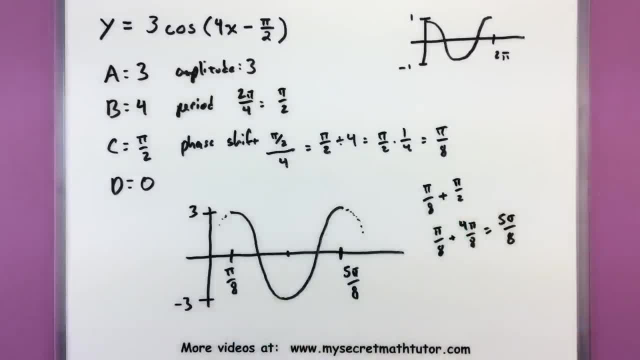 And if I chopped that in half, it'll tell me what I need to add or subtract to figure out that middle point. This middle point is at 3 pi over 8.. The first guy over here is at 2 pi over 8.. 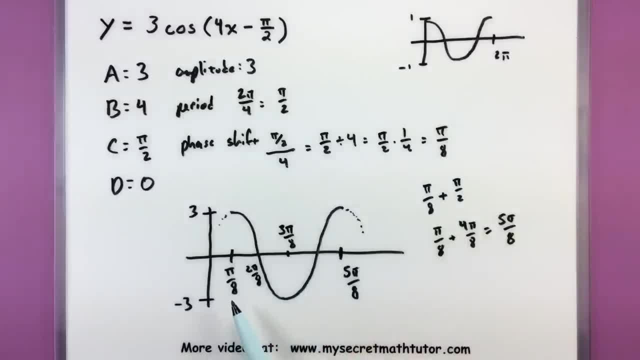 And what I want you to recognize is that I'm essentially going up by 1 8th pi every single time. So 1 8th, 2 8ths, 3 8ths, 4 8ths, 5 8ths. 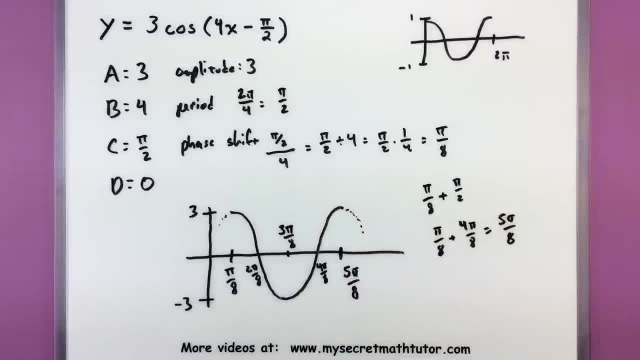 And now we're good to go. Alright, so there's one period of our graph for 3 cosine pi over 8.. Alright, so there's one period of our graph for 3 cosine pi over 8.. Alright, so there's one period of our graph for 3 cosine pi over 8.. 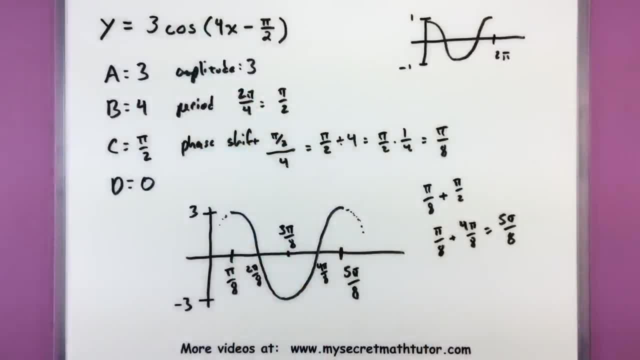 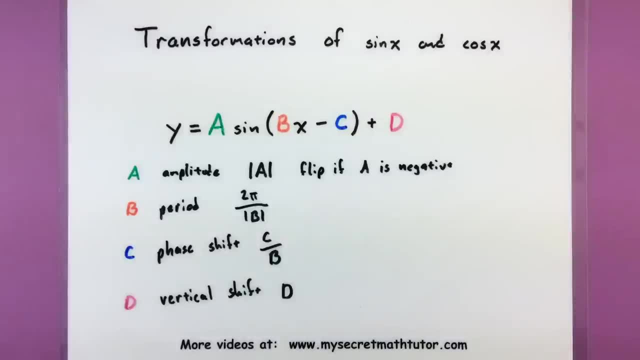 And then we have a sine of 4x minus pi over 2.. Alright, so no matter which graph of sine or cosine you run across, just keep all of those transformations in mind, and you should be good to go. Remember that it's not necessarily the numbers themselves. 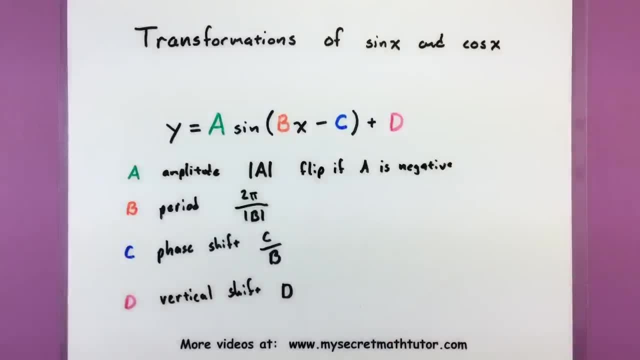 You might have to do a little bit of work to extract the information out from them, but then you should be good. If you'd like to see some more videos, please visit MySecretMathTutorcom.